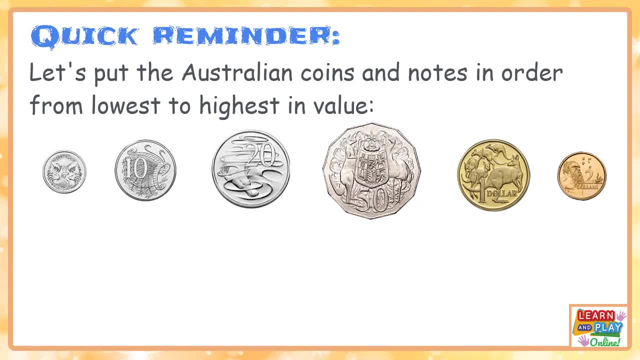 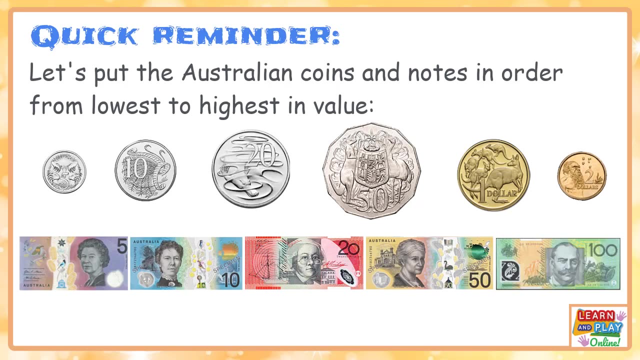 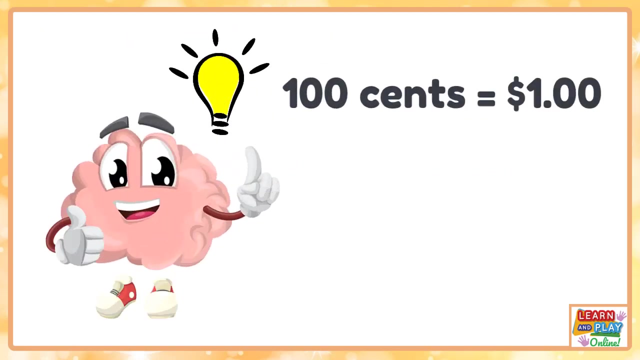 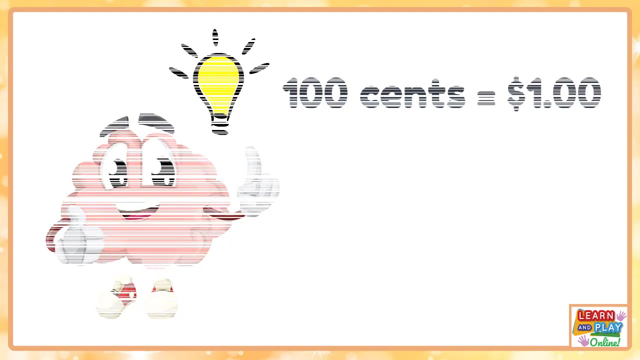 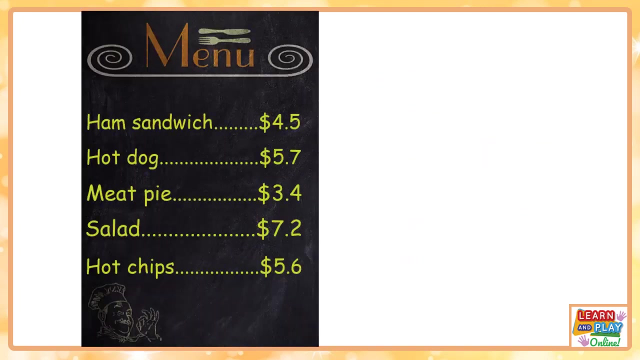 One dollar, Two dollars, Five dollars, Ten dollars, Twenty dollars, Fifty dollars, One hundred dollars. Also, don't forget that there are one hundred cents in one dollar. Calculating change can be a difficult thing to do, so let's practice with some questions using a canteen menu. 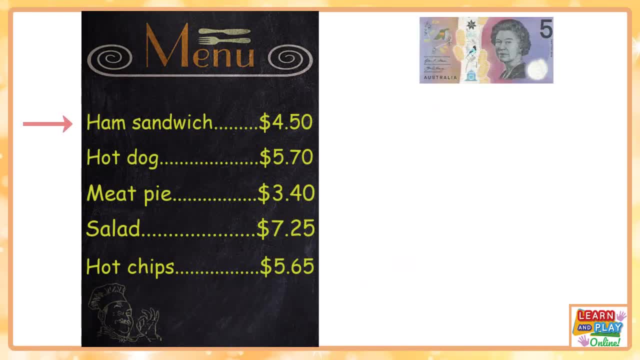 Let's say I have five dollars to spend. If I bought a ham sandwich, how much change would I get back? The ham sandwich will cost me four dollars and fifty cents. Let's separate the dollars and cents to make it easier for us to work out the problem. 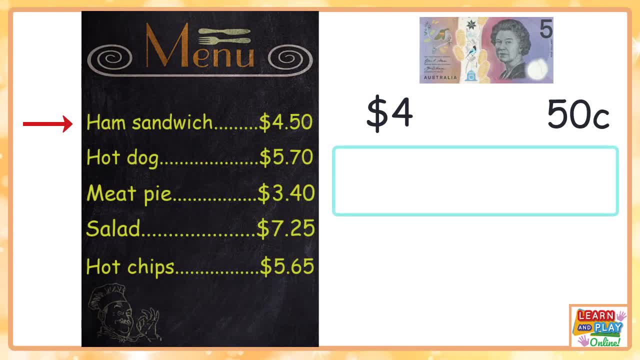 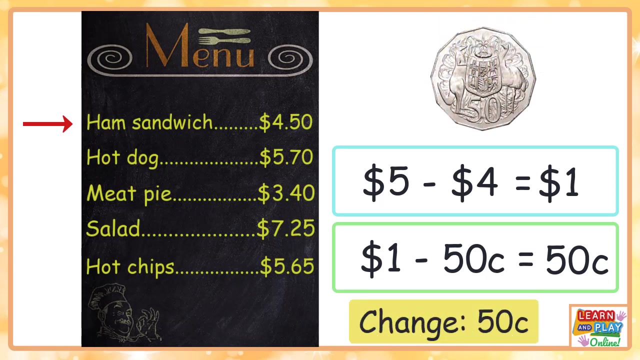 So let's first take away the dollar value: Five dollars. take away four dollars equals one dollar. Now let's work with the cents. One dollar minus fifty cents will leave us with fifty cents. That means we will get fifty cents change. Let's move on to the next one. 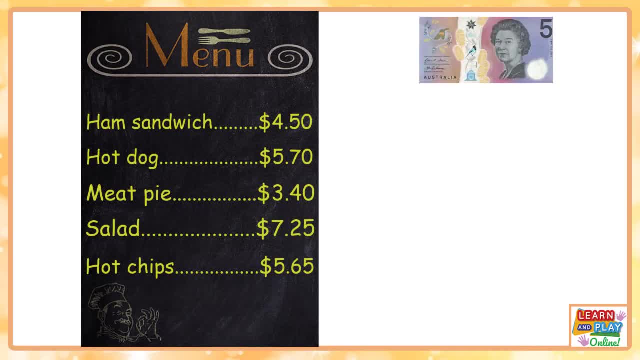 Let's say I start with five dollars once again, but this time I'm going to buy a meat pie. The meat pie is three dollars and forty cents. Again, let's separate the dollars and the cents. Starting with the dollars, let's calculate five dollars minus three dollars. 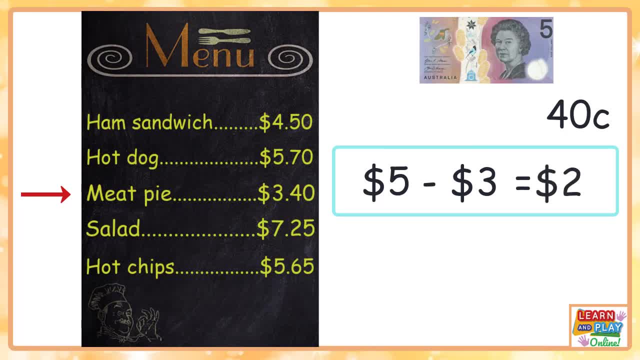 That will leave us with two dollars. Now we're going to work with the cents. Starting with two dollars, we're going to take away forty cents. That will leave us with one dollar and sixty cents. So our change will be one dollar and sixty cents if we buy the meat pie. 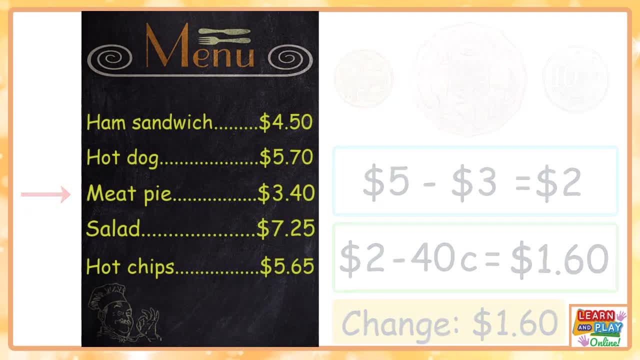 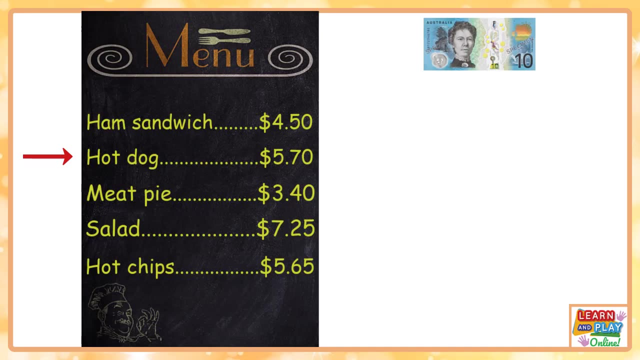 For the rest of the choices on the menu, I'm going to pretend that I'm starting with ten dollars. Now let's say I buy a hot dog. As you can see on the menu, the hot dog will cost me five dollars and seventy cents. 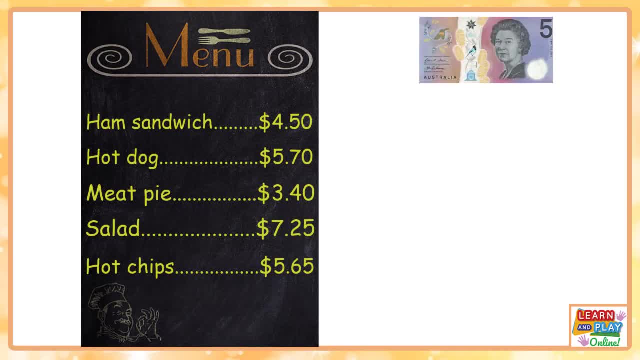 Let's say I start with five dollars once again, but this time I'm going to buy a meat pie. The meat pie is three dollars and forty cents. Again, let's separate the dollars and the cents. Starting with the dollars, let's calculate five dollars minus three dollars. 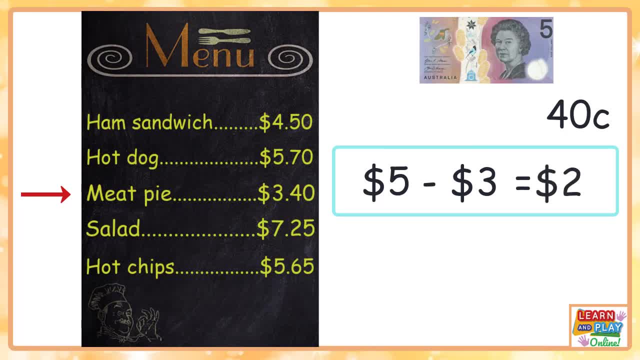 That will leave us with two dollars. Now we're going to work with the cents. Starting with two dollars, we're going to take away forty cents. That will leave us with one dollar and sixty cents. So our change will be one dollar and sixty cents if we buy the meat pie. 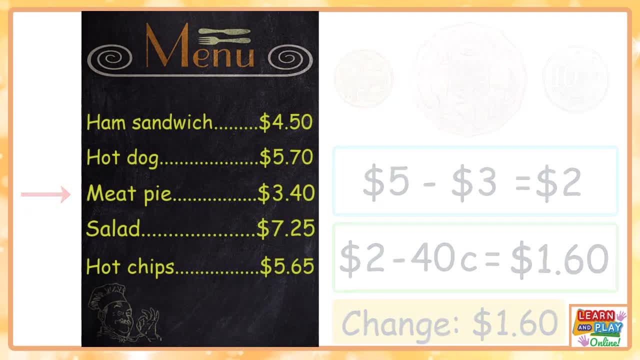 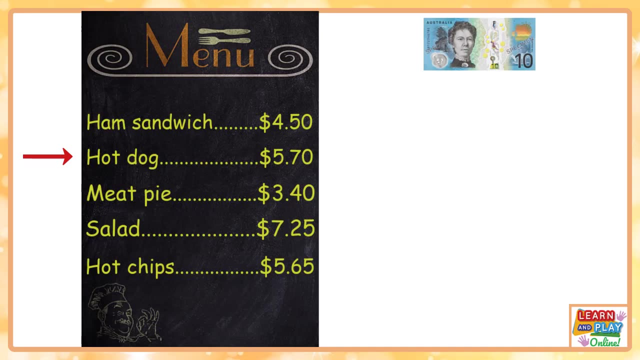 For the rest of the choices on the menu, I'm going to pretend that I'm starting with ten dollars. Now let's say I buy a hot dog. As you can see on the menu, the hot dog will cost me five dollars and seventy cents. 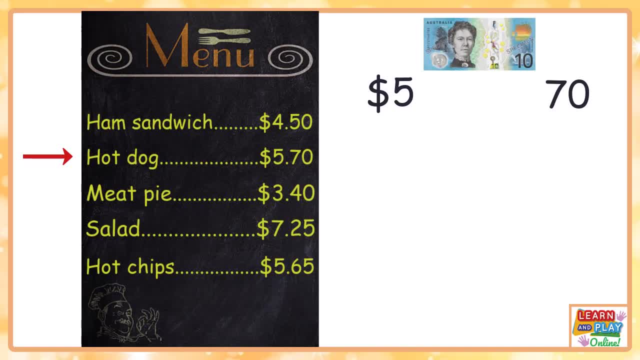 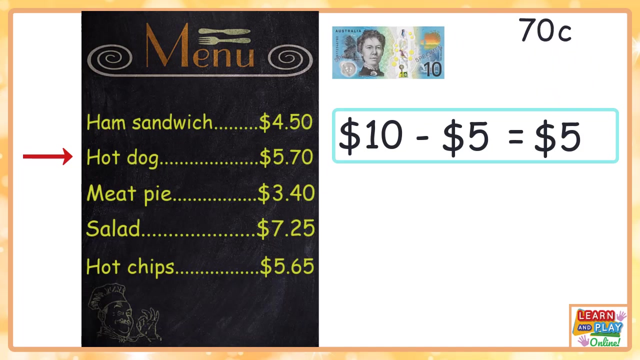 Again, let's separate the dollars and the cents. Starting with the dollars, I'm going to calculate ten dollars minus five dollars. That will leave us with five dollars. Now for the cents. I'm going to try something different: To make seventy cents. I know that I need to have fifty cents plus twenty cents. 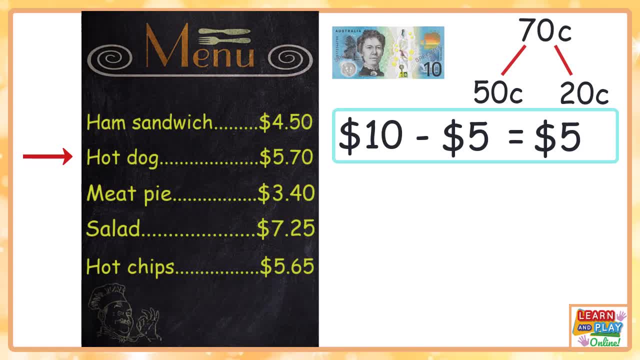 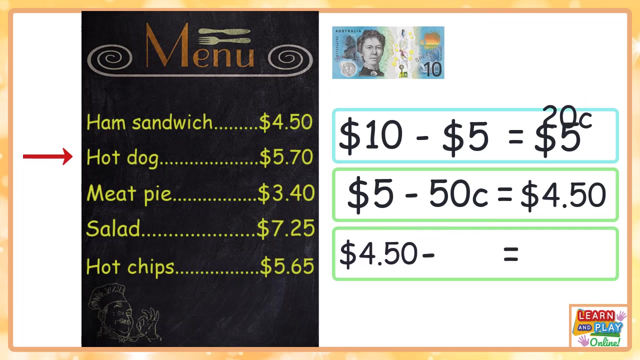 Breaking up the cents even further like this might be a strategy that can help you to subtract cents a little bit easier. Now, starting with my five dollars, I'm going to subtract fifty cents. That will leave me with four dollars and fifty cents. Now we can move on to four dollars, fifty, take away twenty cents. 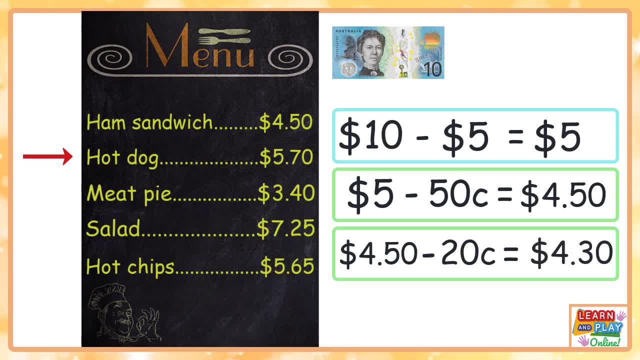 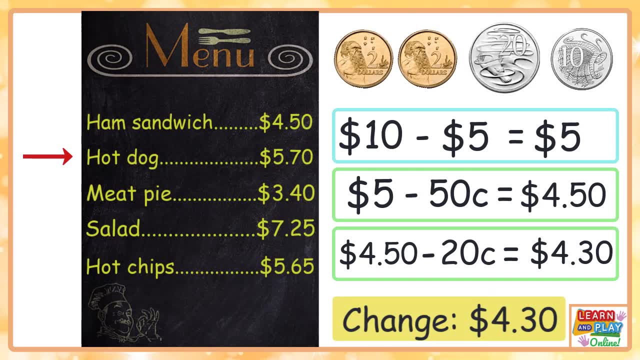 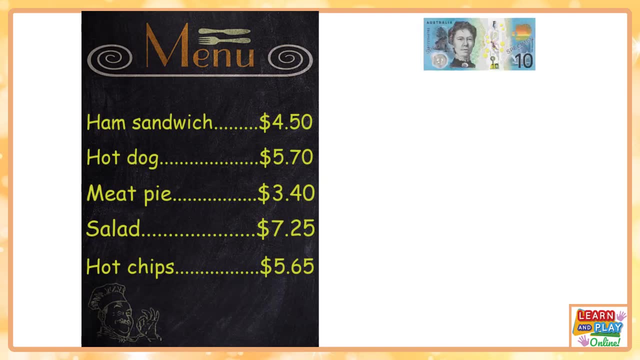 That will leave me with four dollars and thirty cents. So I would get four dollars and thirty cents change if I buy a hot dog. that was five dollars seventy using a ten dollar note. Now let's calculate the change I would receive if I bought hot chips for five dollars and sixty-five cents with a ten dollar note. 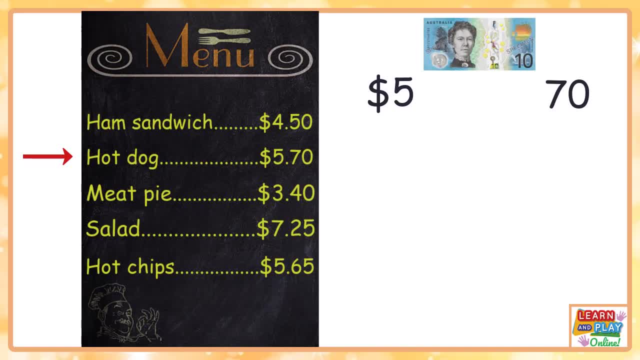 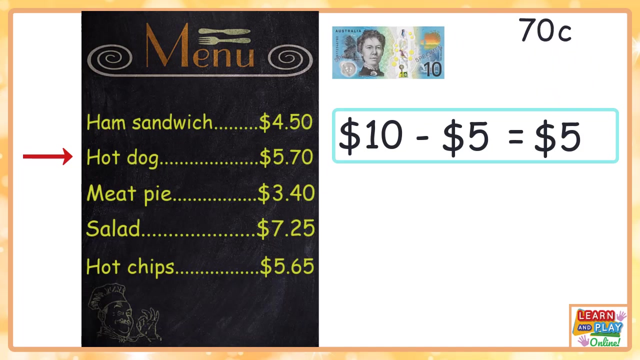 Again, let's separate the dollars and the cents. Starting with the dollars, I'm going to calculate ten dollars minus five dollars. That will leave us with five dollars. Now for the cents. I'm going to try something different: To make seventy cents. I know that I need to have fifty cents plus twenty cents. 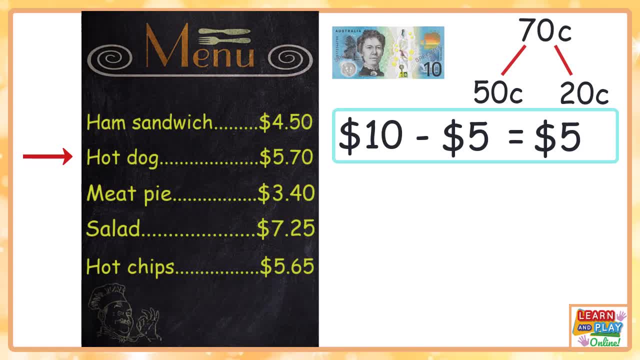 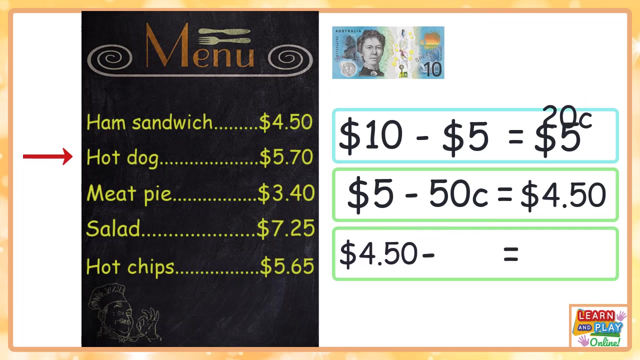 Breaking up the cents even further like this might be a strategy that can help you to subtract cents a little bit easier. Now, starting with my five dollars, I'm going to subtract fifty cents. That will leave me with four dollars and fifty cents. Now we can move on to four dollars, fifty, take away twenty cents. 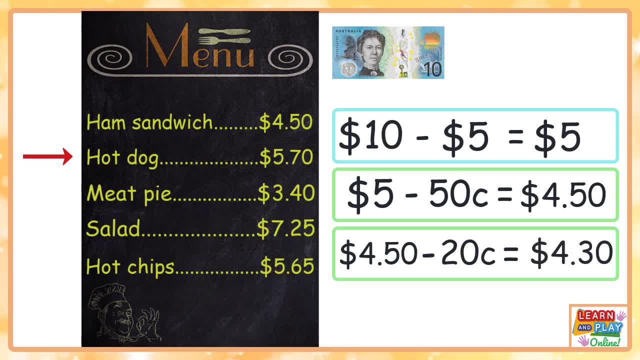 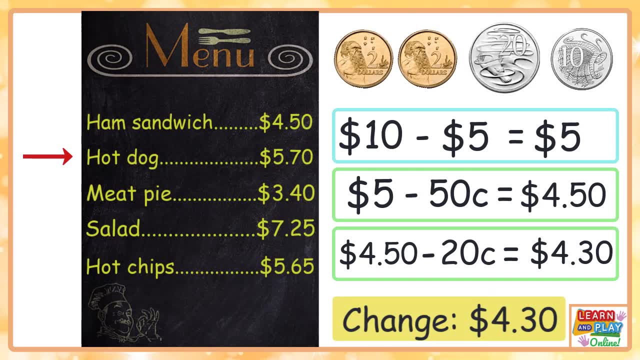 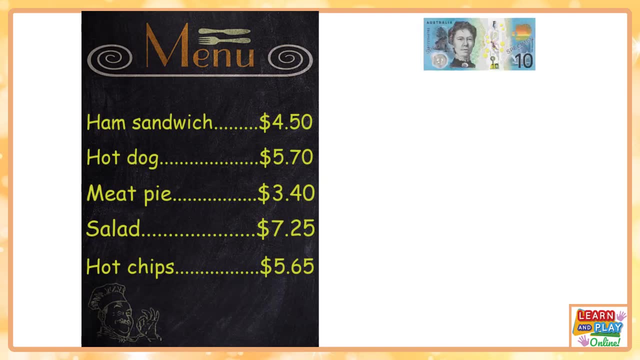 That will leave me with four dollars and thirty cents. So I would get four dollars and thirty cents change if I buy a hot dog. that was five dollars seventy using a ten dollar note. Now let's calculate the change I would receive if I bought hot chips for five dollars and sixty-five cents with a ten dollar note. 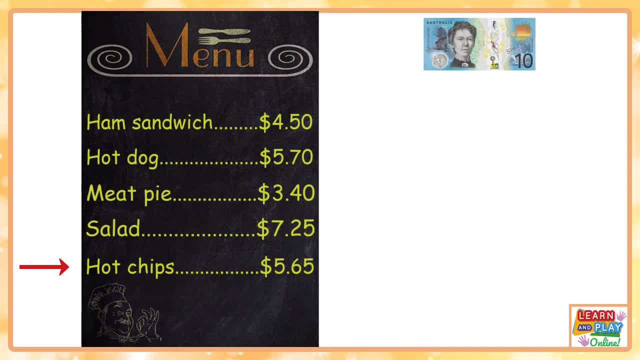 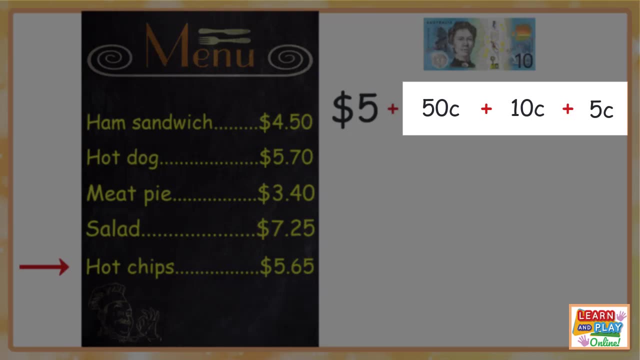 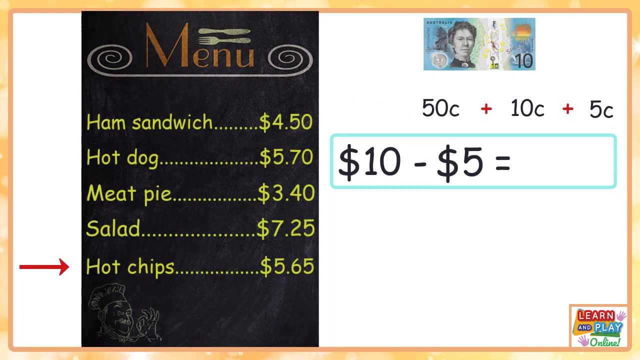 I'm going to represent five dollars and sixty-five cents, with five dollars plus fifty cents, plus ten cents plus five cents, because I know that these amounts here will give me a total of sixty-five cents. So, starting with the dollars, ten dollars minus five dollars equals five dollars. 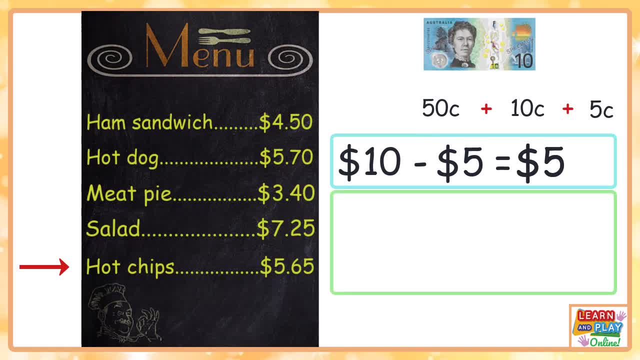 Now to subtract the cents, Five dollars minus fifty cents will leave me with four dollars and fifty cents. Now we work out: four dollars fifty. take away ten cents. That will leave us with four dollars and forty cents. Now, finally, we are left with four dollars forty. take away five cents. 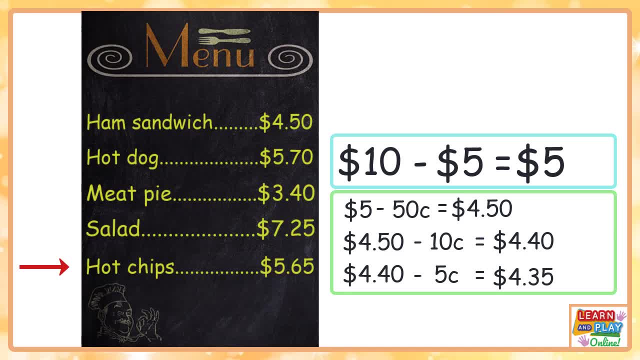 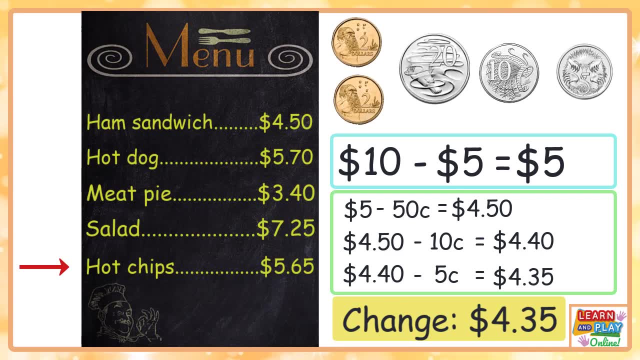 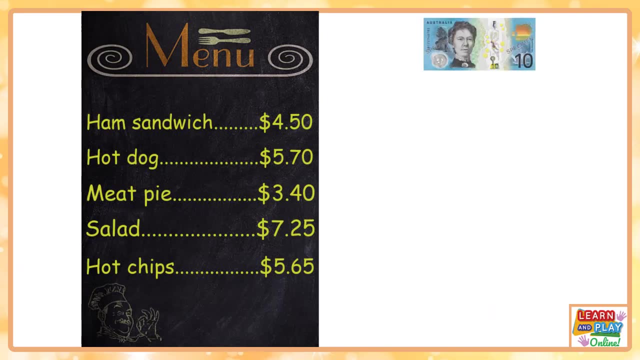 Which is four dollars and thirty-five cents. So we will get change of four dollars and thirty-five cents. Now on to our last problem, Starting with ten dollars. again. this time I'm going to pretend that I'm buying a salad for seven dollars and twenty-five cents.